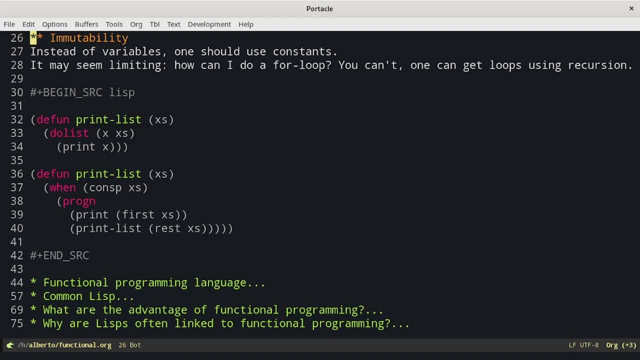 one should use constant whenever it is possible. It may seem limiting. How can I do a for loop? You can't. One gets loops using recursion, For example. here we have two different implementations of a function: printList, that print the element of a list, one per line. In the first case we use directly the doList form. 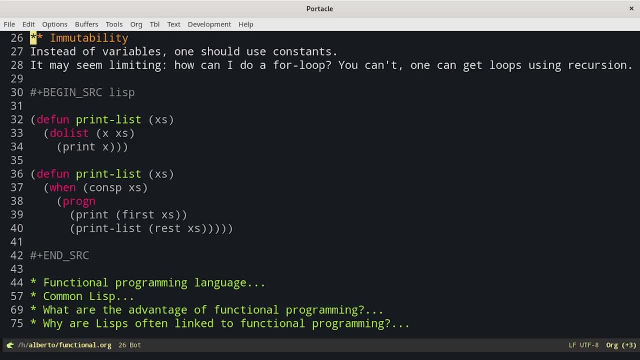 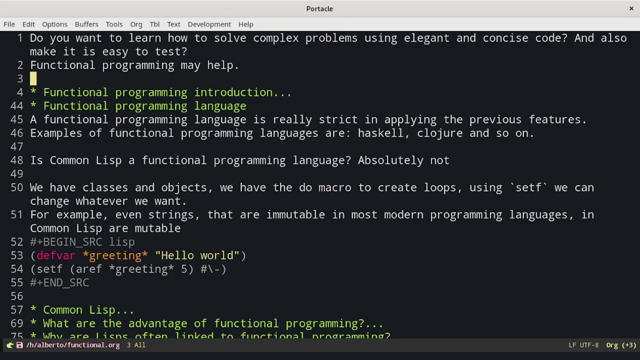 while in the second one we get the loop using recursion. If it is not a cons, for example if it is nil, I do nothing Otherwise. I print the current element and then I continue the recursion on the rest of the list. A functional programming language is really strict in applying the previous features. 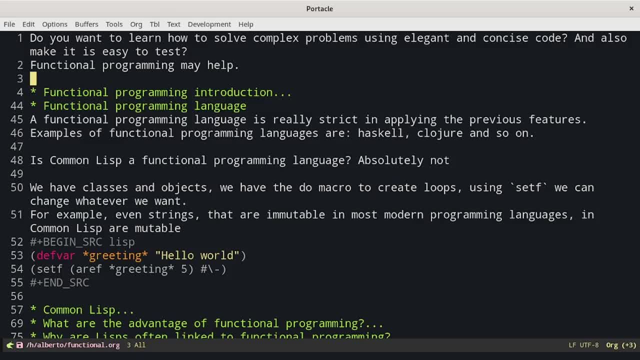 Examples of functional programming languages are Haskell, Clojure and so on. Is Common Lisp a functional programming language? In general, it is not. We have classes and objects. We have the do macro to create loops Using setf. we can change whatever we want, For example even strings that are immutable. 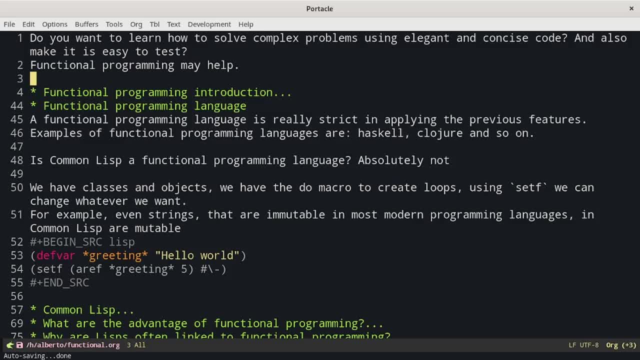 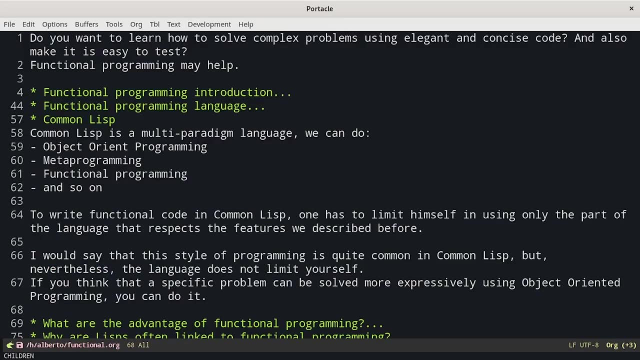 in most modern programming languages. in Common Lisp are mutable. We can define a variable readings, such as Mach and B1, and change one of its characters. Nice and smart, isn't it? Common Lisp is a multi-paradigm language. We can do object-oriented programming. 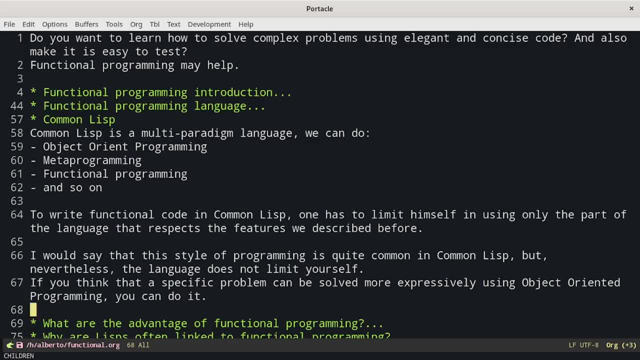 meta-programming, functional programming and so on. To write a functional code in Common Lisp, one has to limit himself in using only the part of the language that respects the features we described before. I was surprised but say that this style of programming is quite common in Common Lisp, but nevertheless. 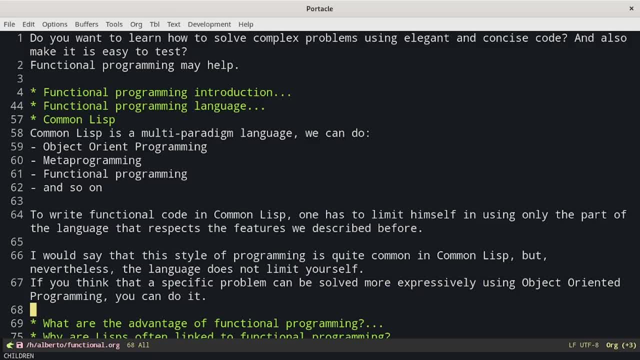 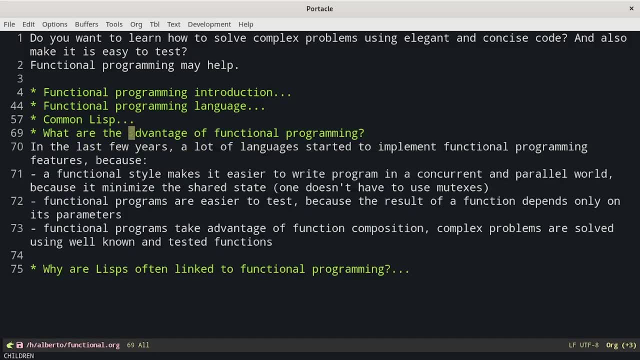 the language does not limit yourself. If you think that a specific problem can be solved more expressively using object-oriented programming, you can do it. What are the advantages of functional programming? In the last few years, a lot of languages started to implement functional programming features because a functional style make